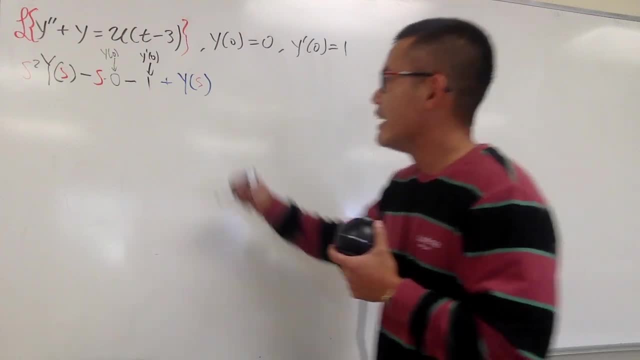 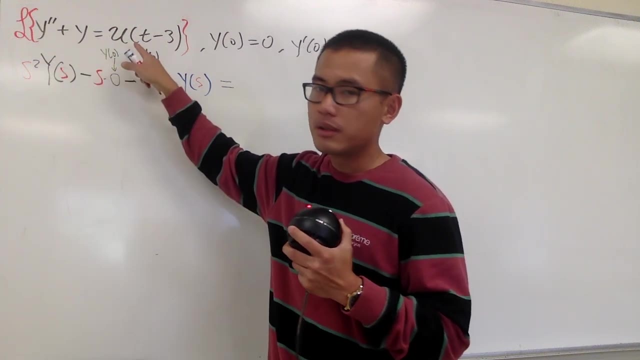 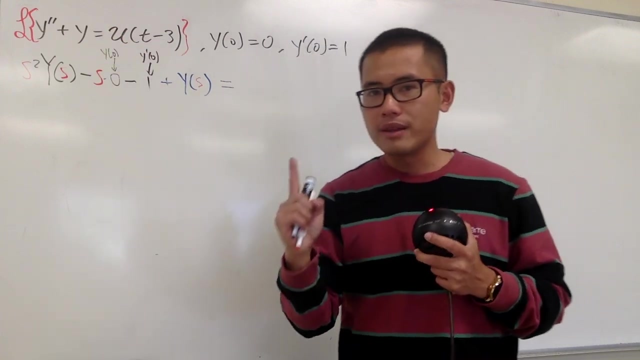 And once again, all my S are in red. all right, And this is equal to the right-hand side. All right, when we do the Laplace transform of the unit step function, as you know, this is technically 1 times U of this. so figure out what's the Laplace transform of 1, which is going to be 1 over S right. 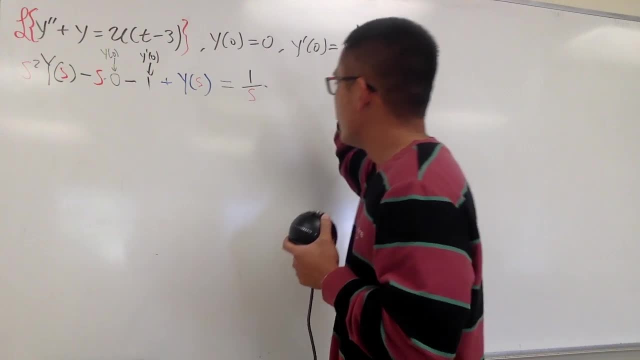 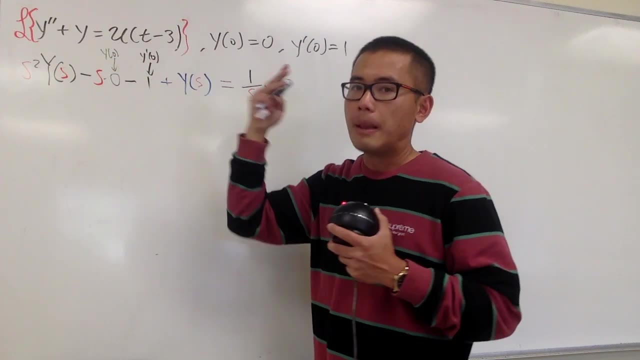 So let's multiply 1 over S, and then we are going to have what? Well, this is U of T minus 3, the positive 3 is what we need, right? So we will have 1 over S times E to the negative 3.. 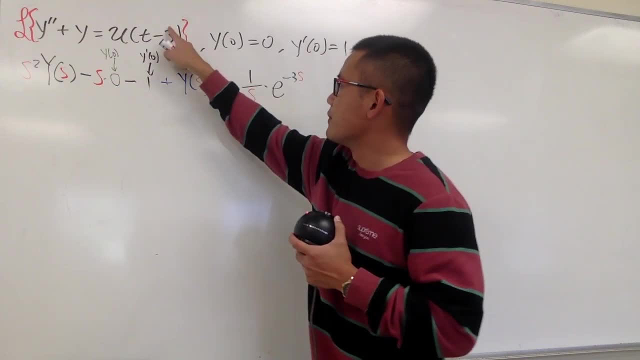 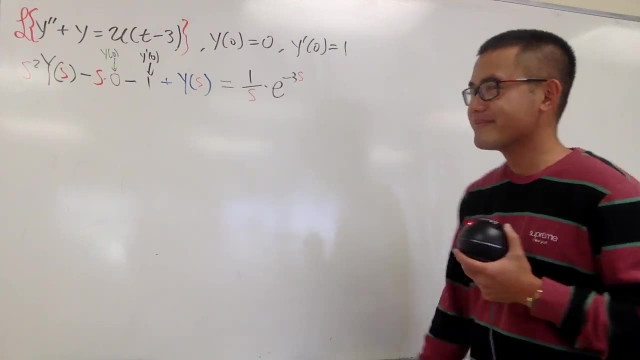 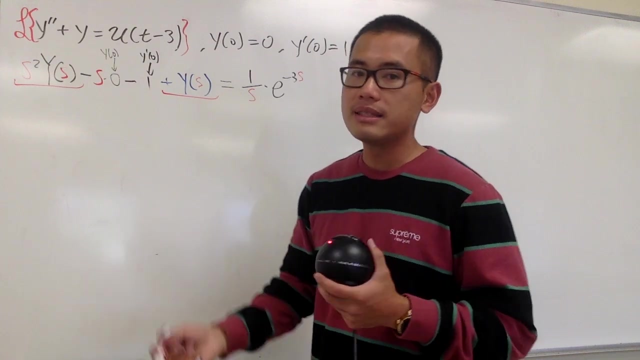 3S. Once again, this 3 is because of minus the 3.. So this is what we have after we take that equation into the S world. Okay, on the left-hand side we see that we have this term and that term. they both have the Y of S. so I'm going to just put them together. 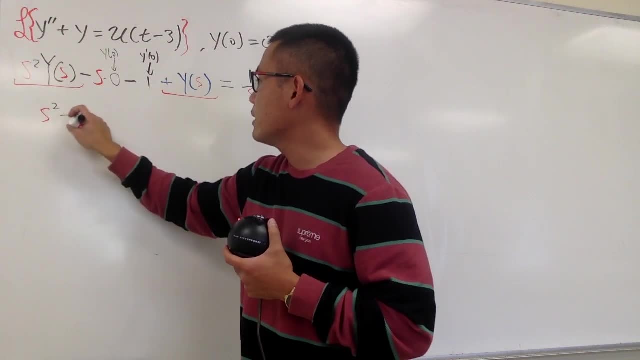 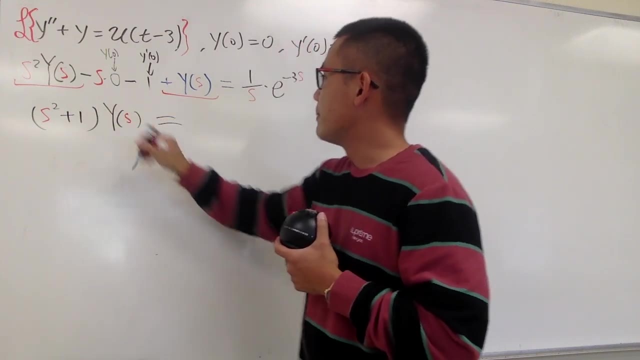 And first we will have the S squared, and then this is plus 1, and then I will factor out the Y of S at the end, like this: And: And this is going to be, and, by the way, this is going to be 0,. so that's it. 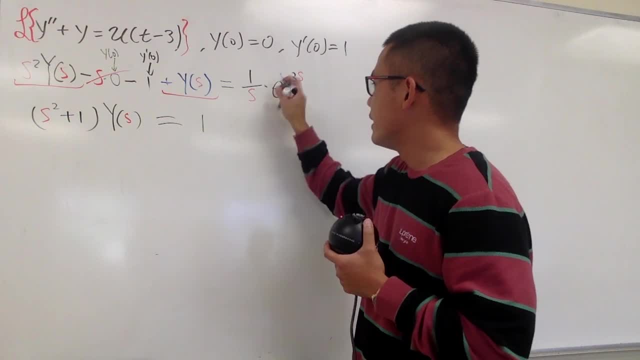 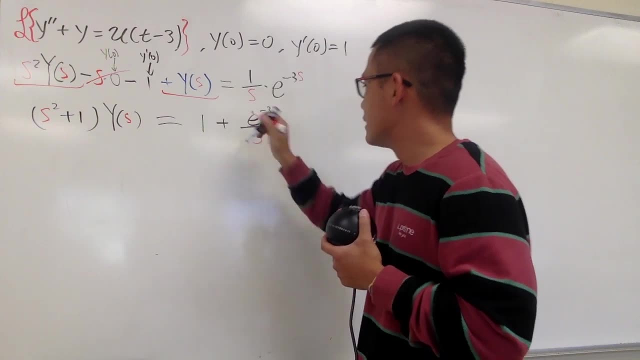 And then bring the 1 to the right-hand side, right, So we will have 1, and then let me put down plus, and let me write this down as E to the negative, 3S over S, And that's what we have. 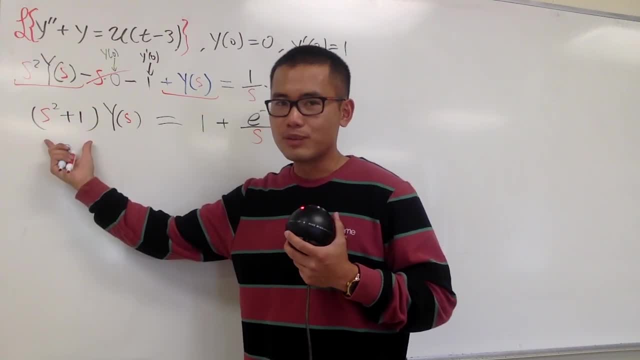 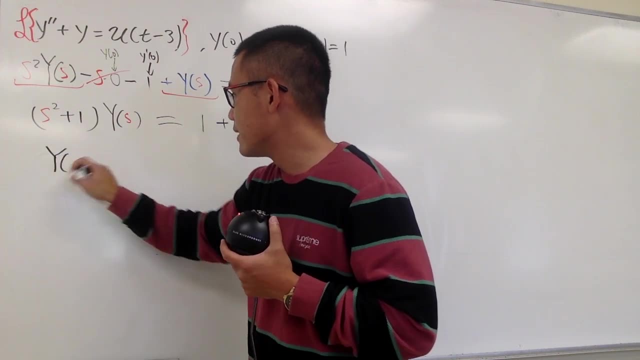 At the end. you know I have to divide everything by S squared plus 1.. In another word, I will get Y of S. This is technically a capital Y, like this Y of S is going to be. First, we have 1 over S squared plus 1.. 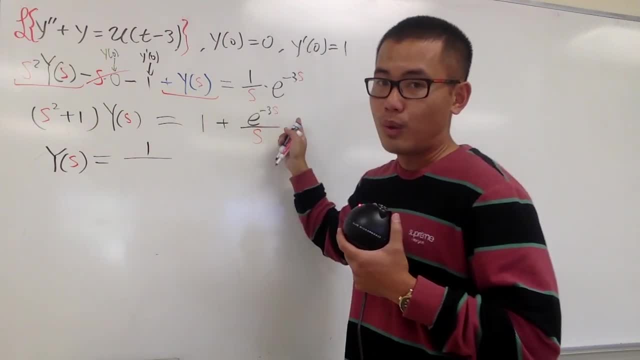 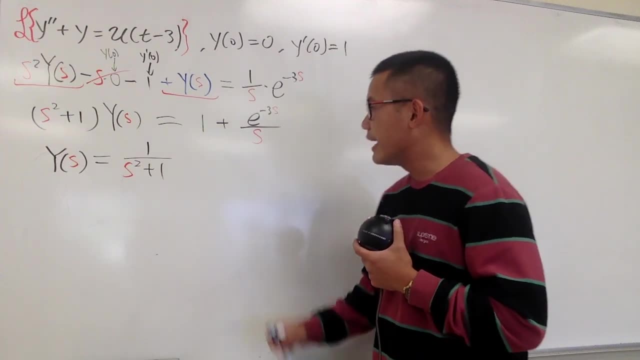 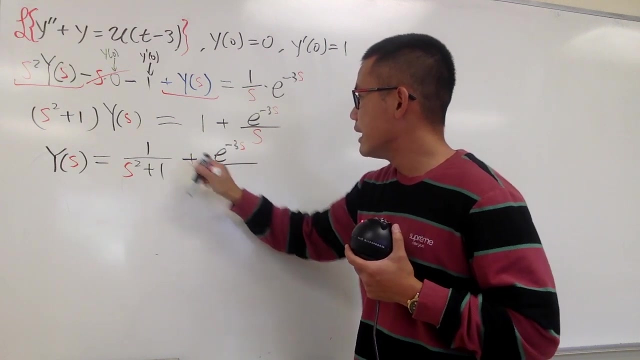 And I'm not going to combine the fractions, because this one doesn't have E to the whatever right. So 1 over S, squared plus 1, okay. And then, right here, we put down plus E to the negative, 3S over S, and then we put this in the denominator, so we have the S squared plus 1, like that okay. 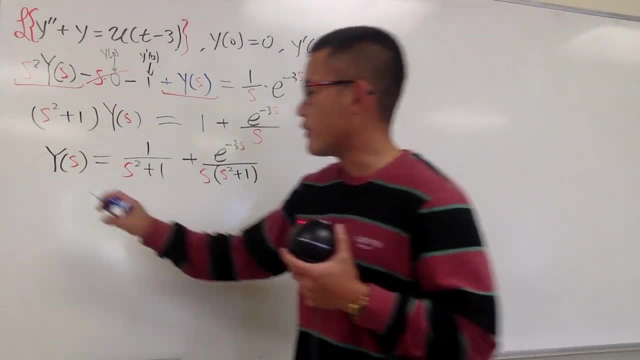 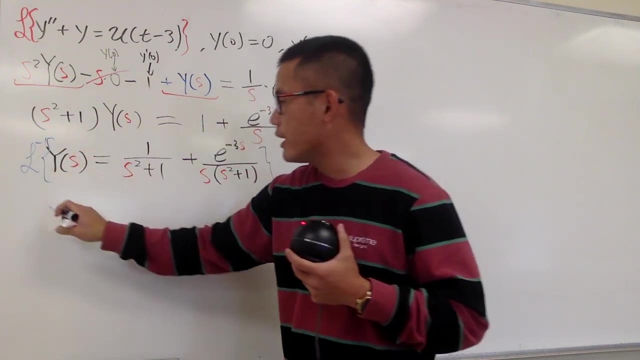 And now, as you know, we will just take the inverse. So let me just do that like this throughout: right, When we go back, we get to the T world, this is going to give us the Y of T, namely, this is going to be the solution, right? 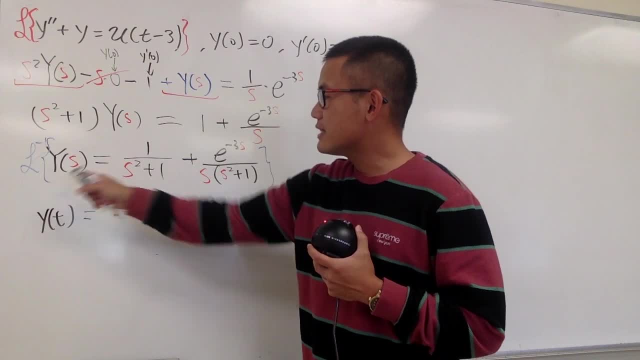 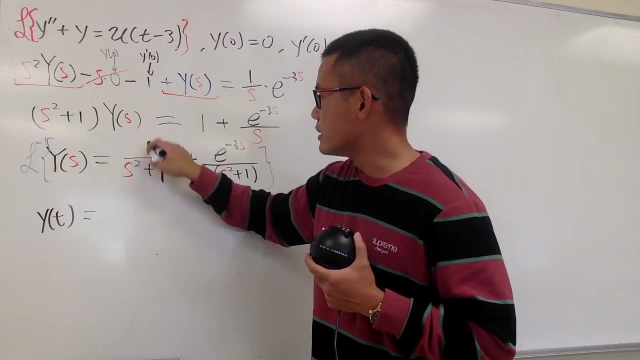 And this is not bad to do, neither The inverse of plus of 1 over S squared plus 1.. This 1 is the same as saying 1 squared and this 1 matches with this 1, right, That means we have what? 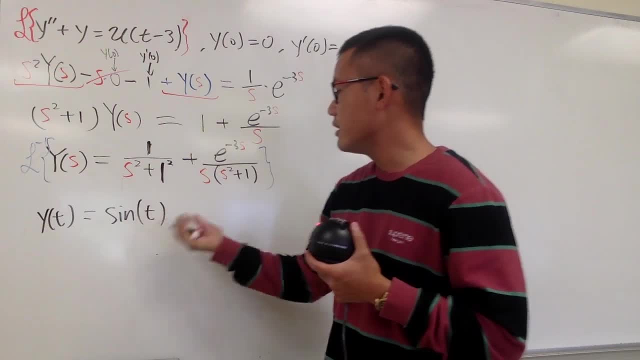 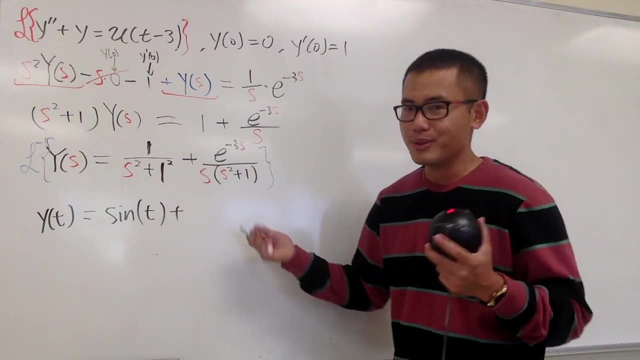 Just sine of 1T, Just sine of 1T, like this. no problem, right. Next we are going to be adding- and this is how you're going to do this: Here we have E- to the negative 3S. 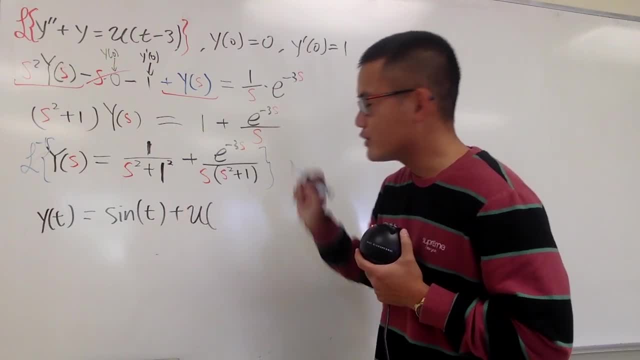 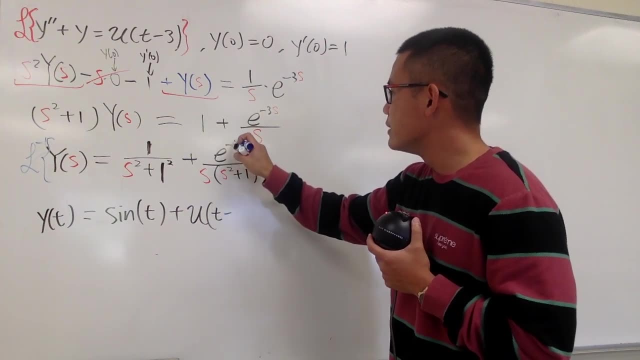 You know, when you go back to the T world, you are going to end up with the unit step function and the input is going to be T minus this 3.. Once again, it's because of negative 3S. So the input is T minus 3, right. 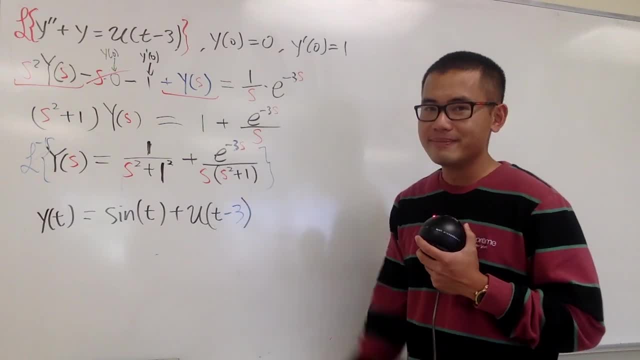 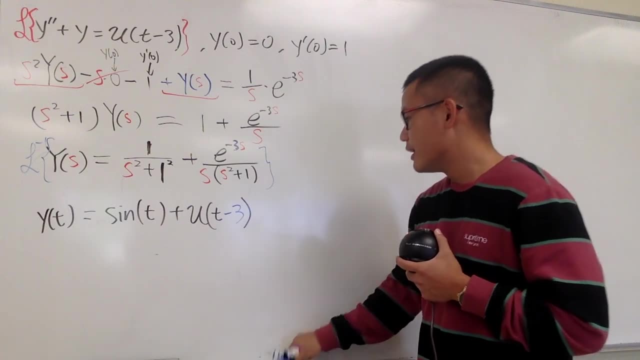 So always You put that down first. whenever you see E to the Y of S. Well, I also have to multiply by F of T minus 3.. That's a zero statement, right? So let me just write this down. 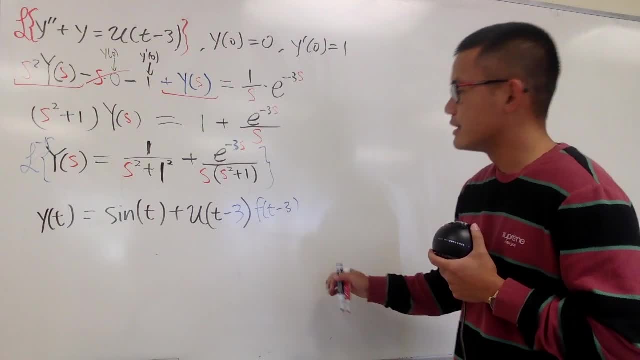 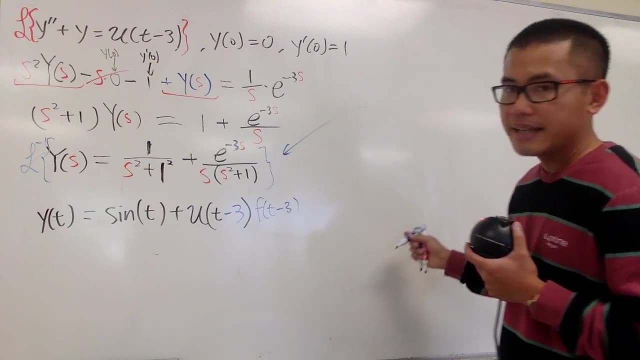 We must have the F of T minus 3 as well. But what's F of T, I don't know yet. So to do so, let me just indicate this on the side: I have to figure out what's the inverse of plus of 1 over. 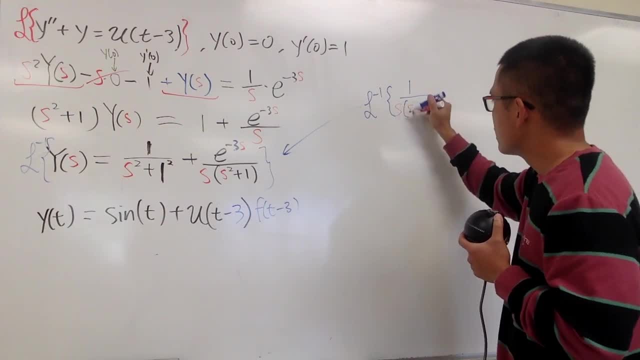 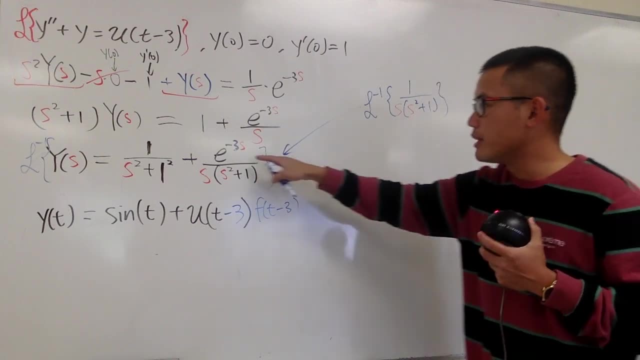 S times S squared plus 1,. all right When you do this. only you see, on the top I did not put down E to the negative 3S anymore, because this right here, by itself it's going to give us F of T. 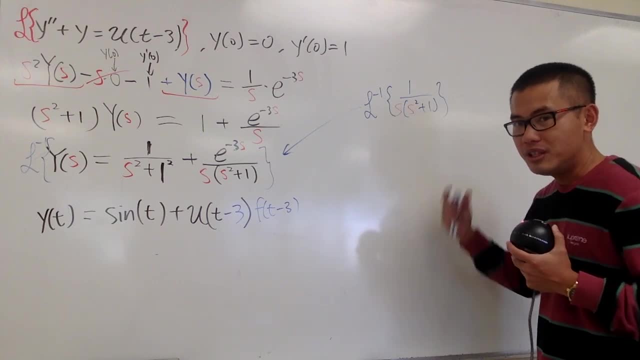 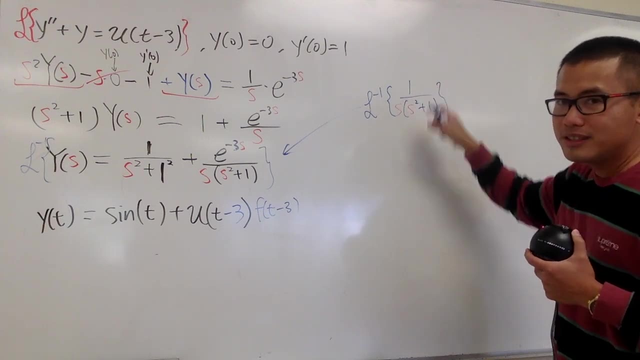 And once I know F of T, I can just plug in T minus 3 into T and then I will figure out this part. So anyway, this is 1 over S times S squared plus 1.. To do this we have to do partial fractions. 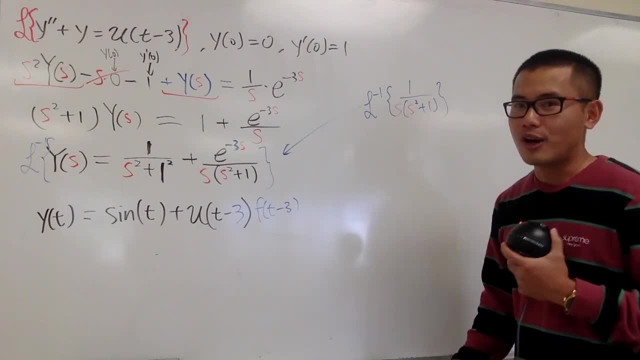 And you can check out the video in the description. And you can check out the video in the description. I'll show you guys how to do a partial fraction in a different video, because I wouldn't have enough space to do all that for you guys right here. 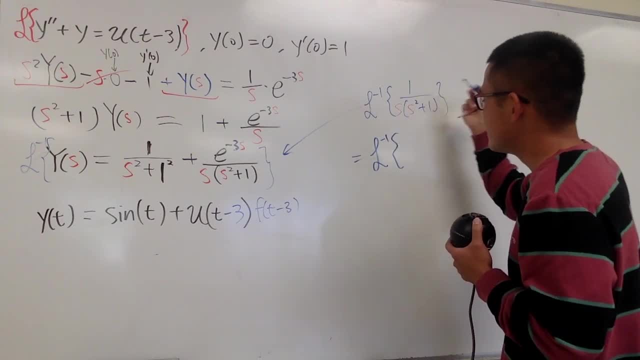 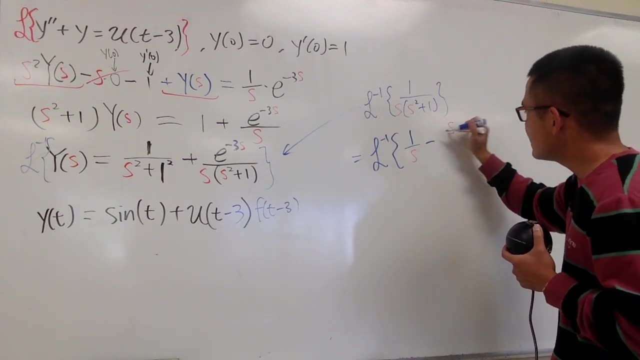 So just please watch the video or, better yet, try this on your own. And either way, you are going to end up with 1 over S, and then you are going to subtract S over S, squared plus 1.. Once again, just by partial fraction. 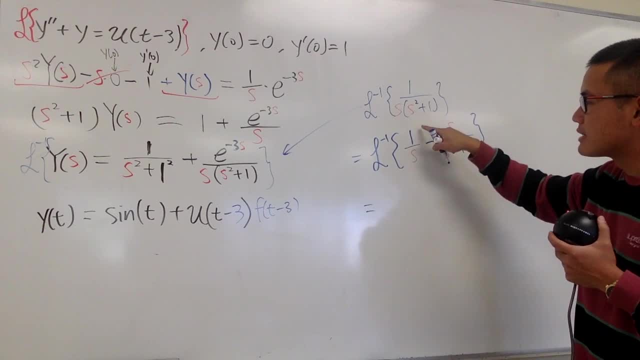 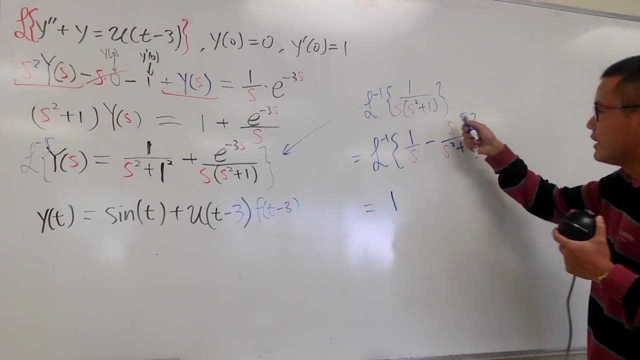 And then now you see, the inverse Laplace of 1 over S is going to be 1.. Because the Laplace of 1 is 1 over S. right For this. as you can see, we have S on the top, S squared on the bottom, like this, and then plus 1, right. 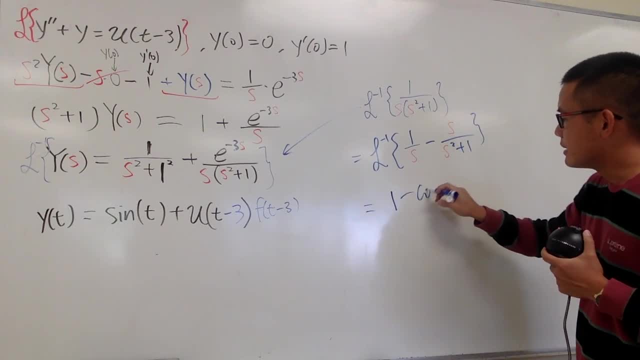 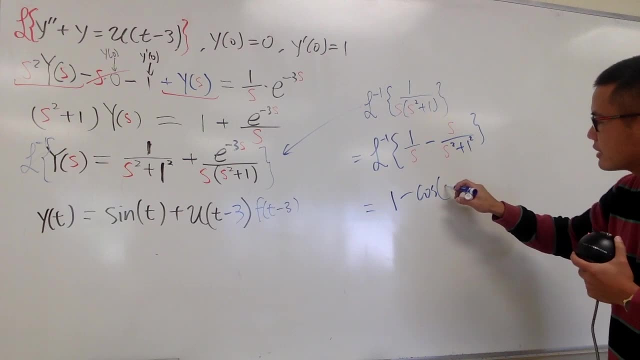 This is going to give us cosine, and then this is a minus, So minus cosine, And this is technically the same as 1 squared right. So in other words, minus cosine, T, just like that, And this guy is the F of T, okay. 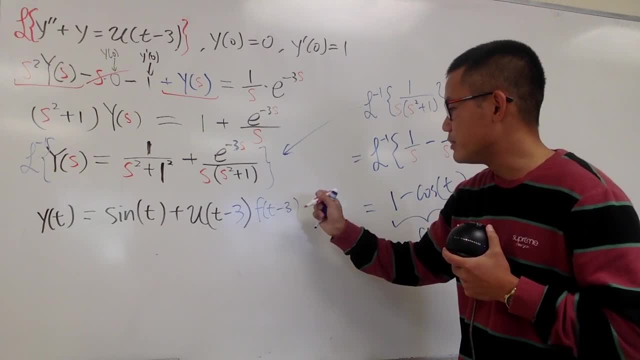 And now I just have to figure out what's F of T minus 3.. And now I just have to figure out what's F of T minus 3.. Let me just indicate that I want the input to be T minus 3.. 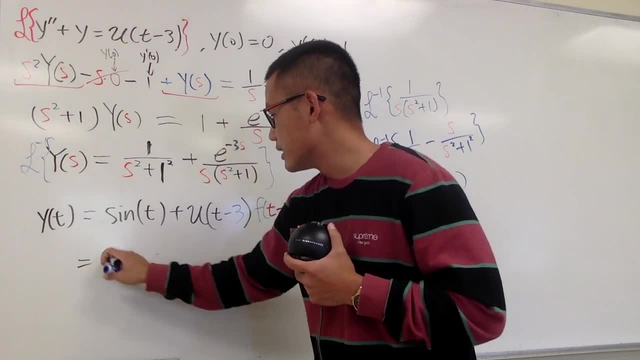 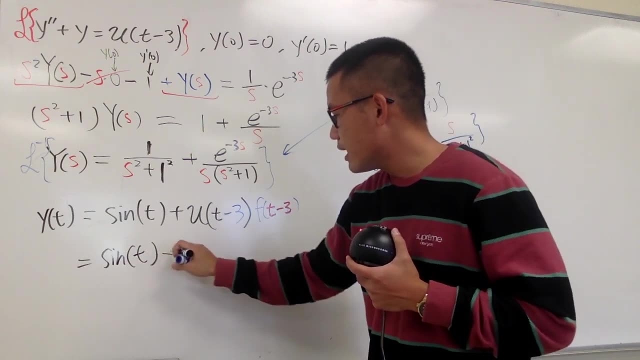 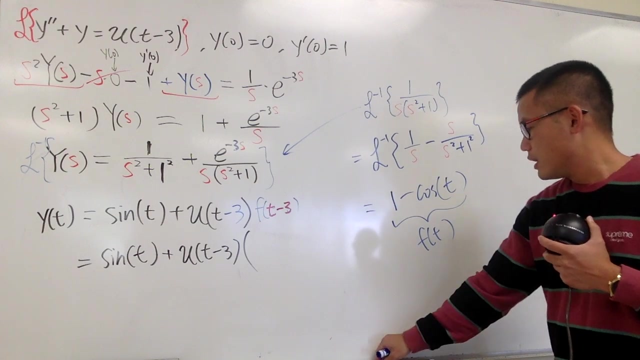 So to write this down legitimately, I will write this down as sine T by itself. right, This is like one term, the first term, And then plus U of T minus 3.. And I open the parentheses for the F of T minus 3.. 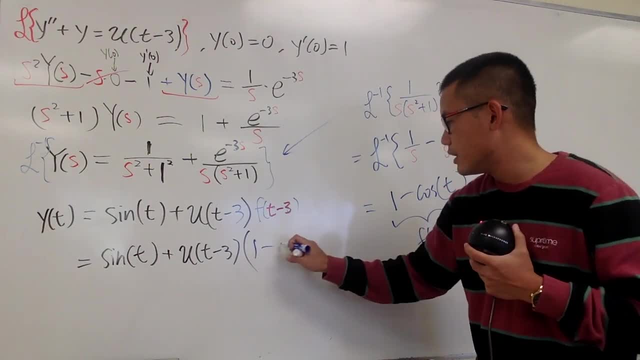 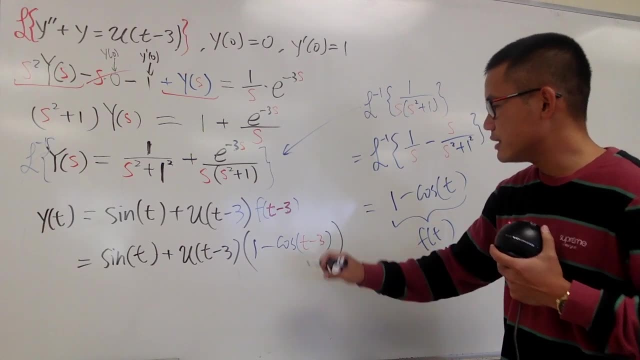 Okay, 1. And then minus cosine, And the T becomes T minus 3.. So put on T minus 3 inside And then close that parentheses. That's it. This right here is the solution, And this is my little letter Y. 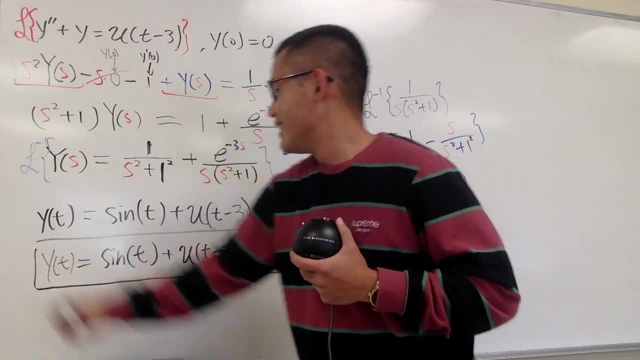 But anyway, it shouldn't matter that much. Anyway, that's it Pretty fun, isn't it? 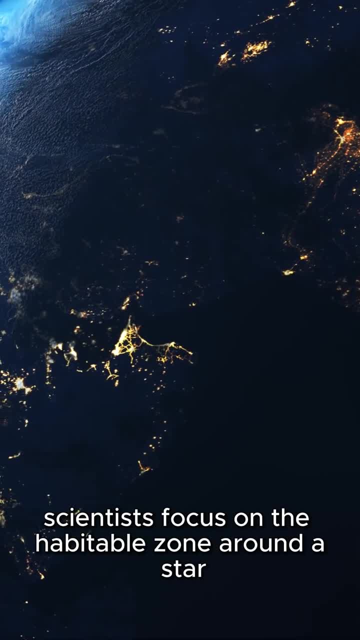 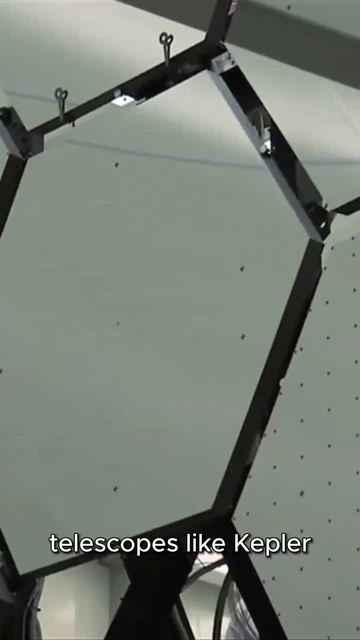 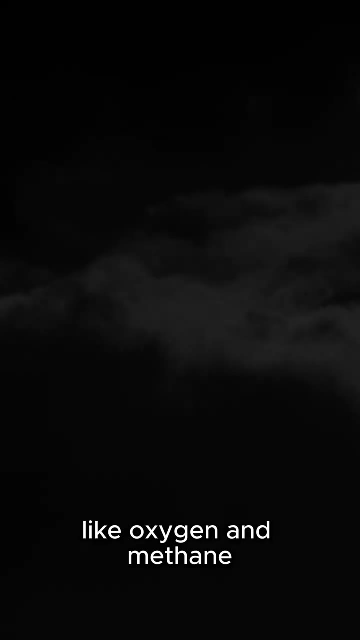 To discover habitable exoplanets. scientists focus on the habitable zone around a star where conditions allow for liquid water. Telescopes like Kepler and the upcoming James Webb Space Telescope analyze atmospheres for potential biosignatures like oxygen and methane.